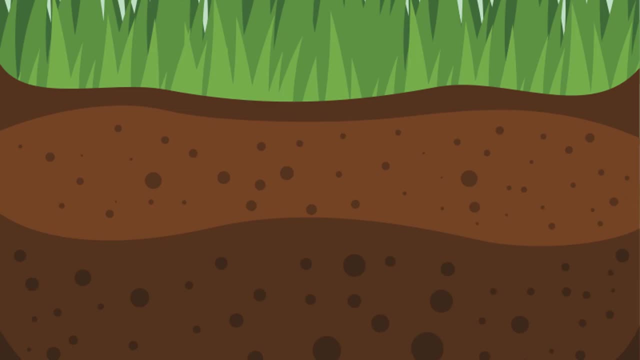 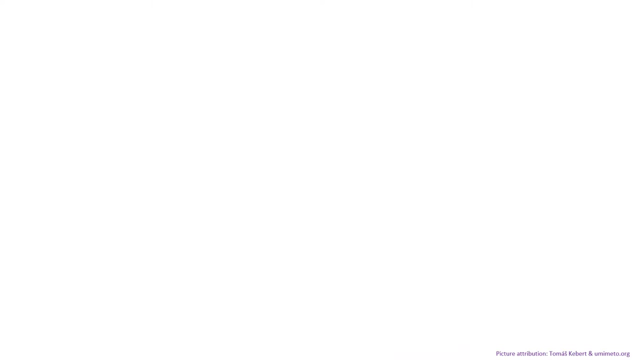 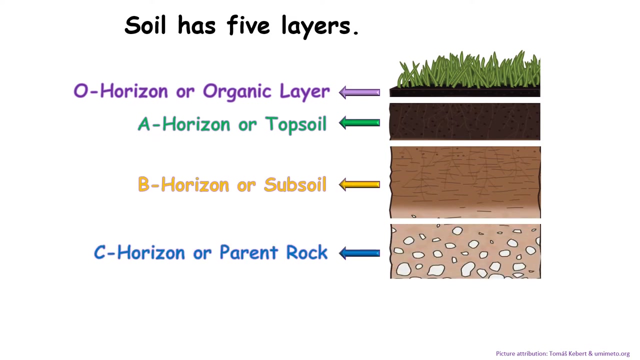 In this video lesson, we will learn about layers of soil. Soil has five layers. They are: O horizon or organic layer. A horizon or topsoil. B horizon or subsoil. C horizon or parent rock. and R horizon or bedrock. 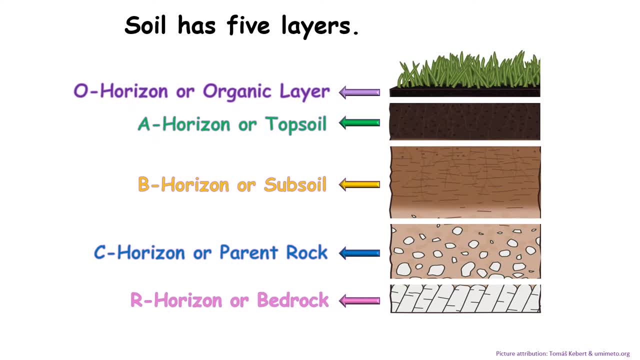 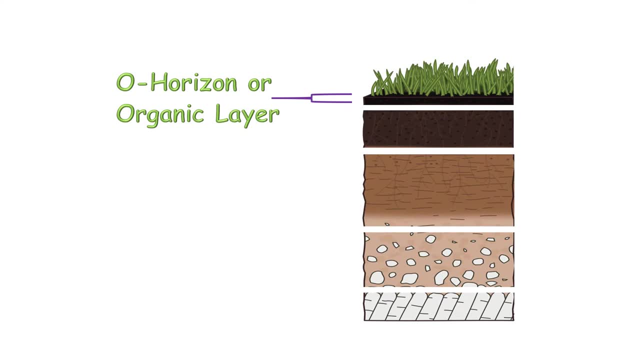 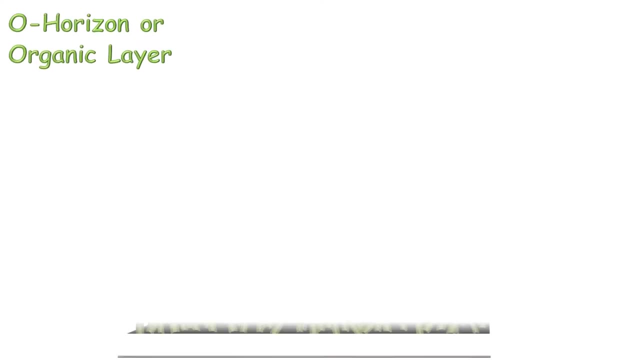 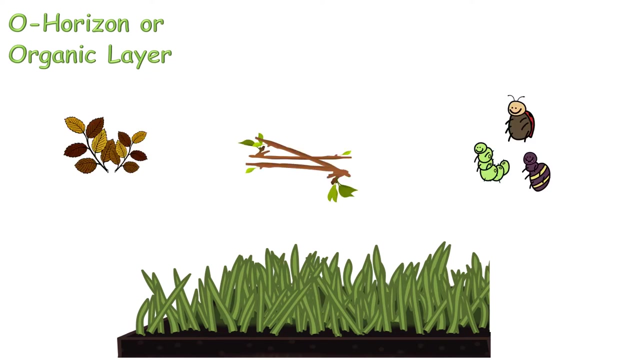 Let's learn about these five layers one by one. O horizon or organic layer. It is the thin, topmost layer. It is a layer of dead plant and animal material, like dead leaves, twigs and insects. This dead material makes O horizon rich in organic matter, also known as humus. 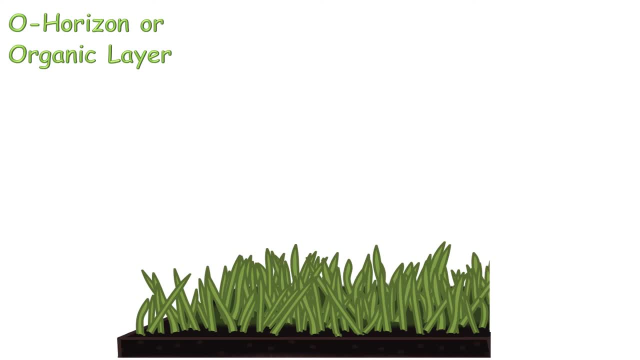 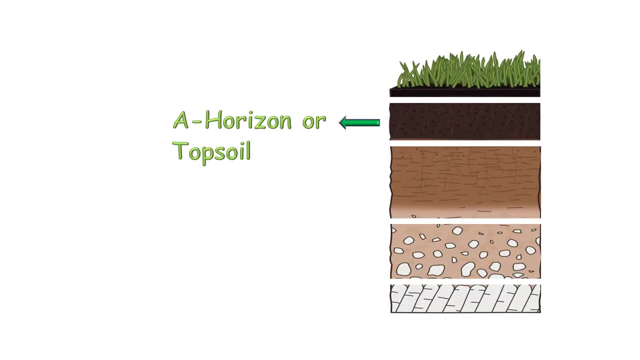 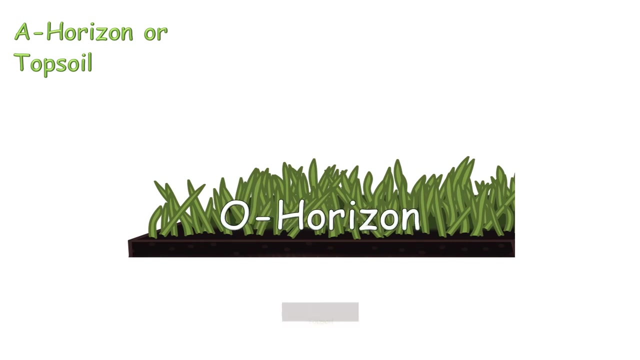 which is helpful for the growth of plants. Organic layer may or may not be present in different land types. The land type that has this layer is the most fertile. A horizon or topsoil. Below O horizon is the A horizon or the topsoil. 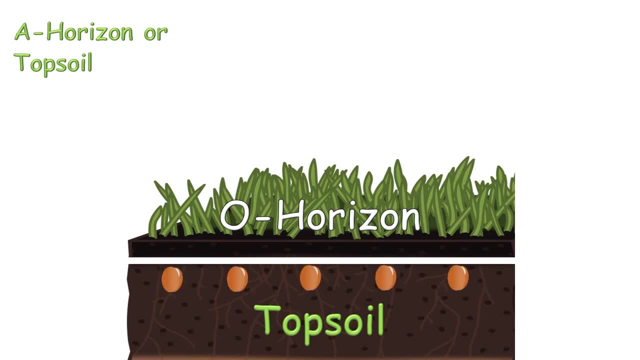 This is the layer where we sow seeds. This layer is rich in humus and minerals. The soil in this layer is soft and porous, so it can hold enough air and water. All these conditions help seeds to germinate and grow into new plants. 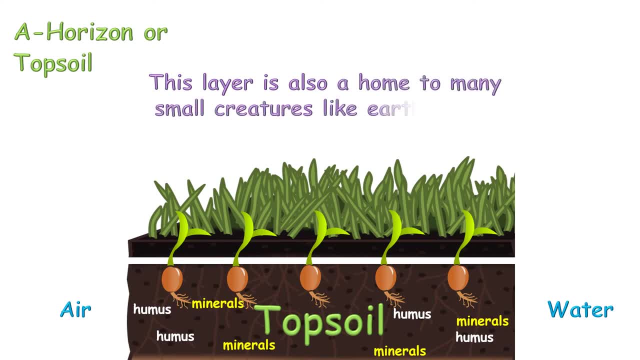 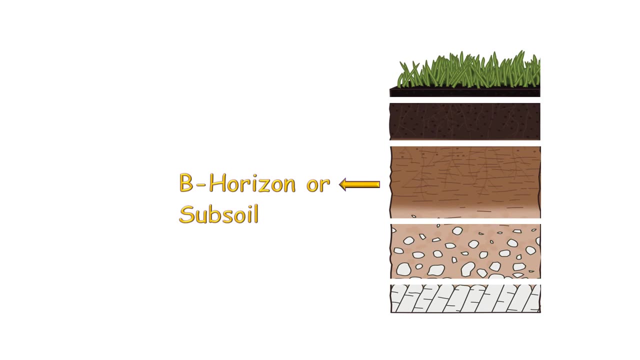 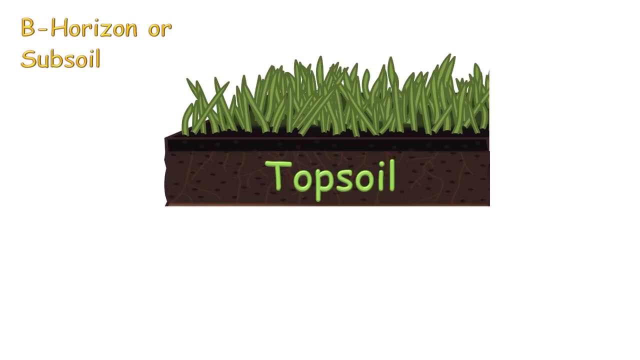 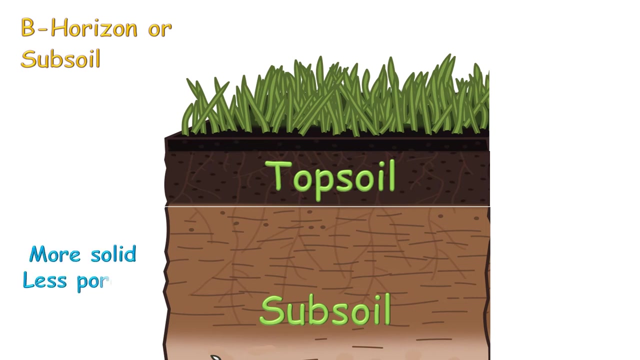 This layer is also a home to many small creatures like earthworms, bugs and microorganisms like bacteria and fungi. Bee Horizon or Subsoil- Below top soil is present. bee horizon or subsoil: This layer is more solid and less porous.